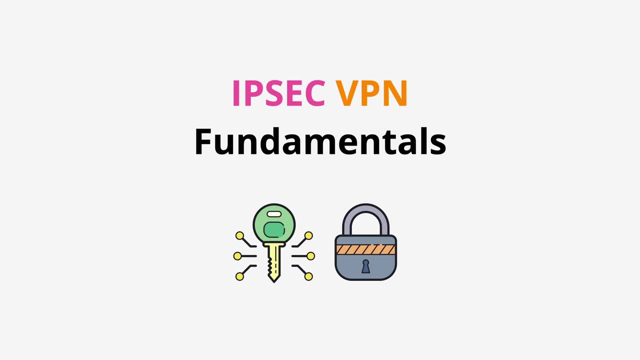 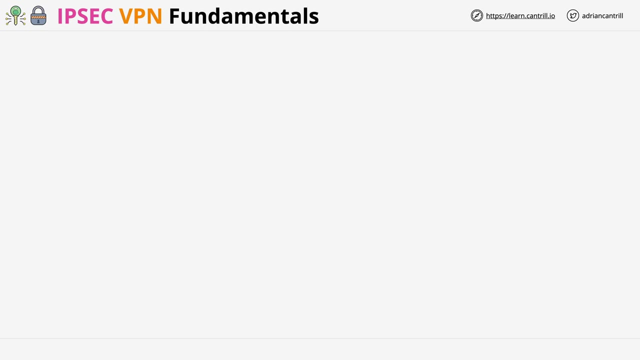 Welcome back and in this lesson I want to cover IPsec fundamentals. So I want to talk about what IPsec is, why it matters and how IPsec works at a fundamental level. Now we have a lot of theory to cover, so let's jump in and get started At a foundational level. 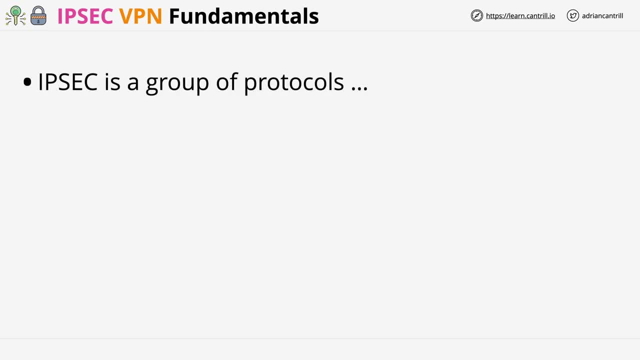 IPsec is a group of protocols which work together. Their aim is to set up secure networking tunnels across insecure networks, For example, connecting two secure networks, or more specifically, their routers, called peers, across the public internet. Now you might use this if you're a. 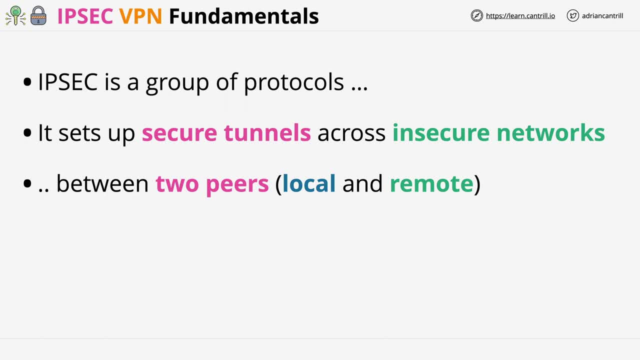 business with multiple sites spread around geographically and want to connect them together, or if you have infrastructure in AWS or another cloud platform and want to connect to that infrastructure. IPsec provides authentication so that only peers which are known to each other and can authenticate their network can connect to each other. So IPsec is a group of protocols. 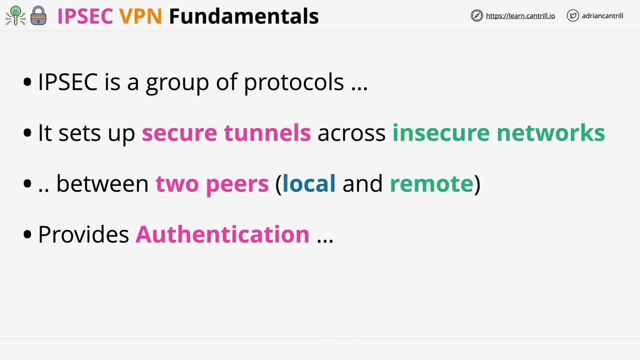 that can authenticate with each other can connect, and any traffic which is carried by the IPsec protocols is encrypted, which means to onlookers the secure data which is being carried is cipher text. It can't be viewed and it can't be altered without being detected. Now, architecturally it 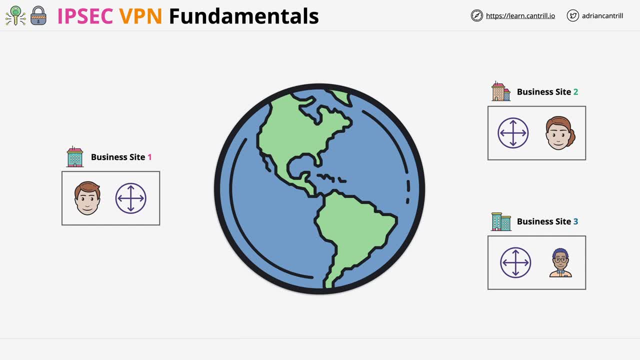 looks like this. We have the public internet, which is an insecure network full of goblins looking to steal your data. Over this insecure network, we create IPsec tunnels between peers. Now these tunnels exist as they're required Within IPsec VPNs. there's the concept. 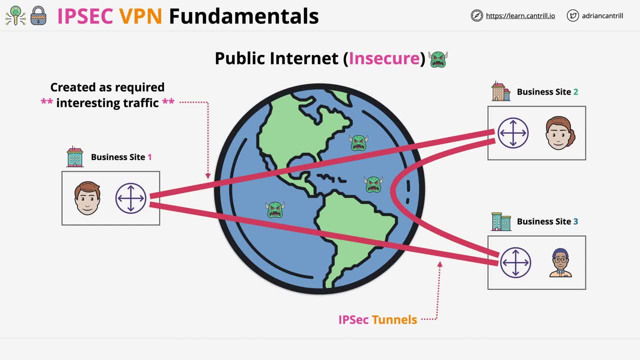 of interesting traffic. Now, interesting traffic is simply traffic which matches certain rules, and these could be based on network prefixes or match more complex traffic types, Regardless of the rules. if data matches any of those rules, it's classified as interesting traffic and a VPN tunnel is created to carry traffic to the IPsec network. Now, if you're a business with multiple sites, 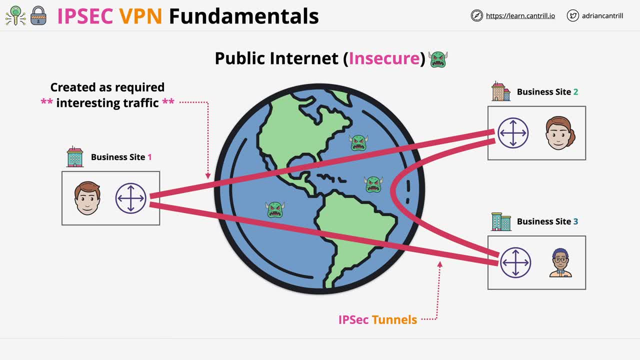 through to its destination. Now, if there's no interesting traffic, then tunnels are eventually torn down, only to be re-established when the system next detects interesting traffic. The key thing to understand is that, even though those tunnels use the public internet for transit, any data within the tunnels is encrypted. while transiting over that insecure network, It's. 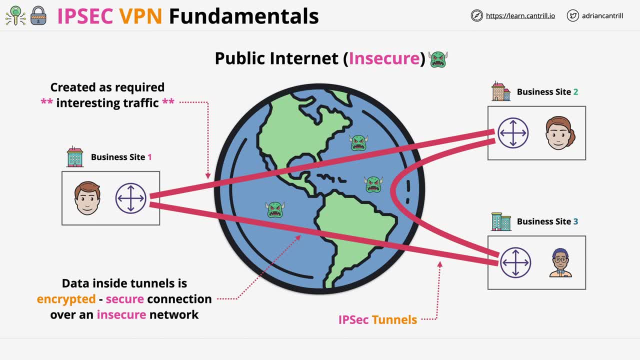 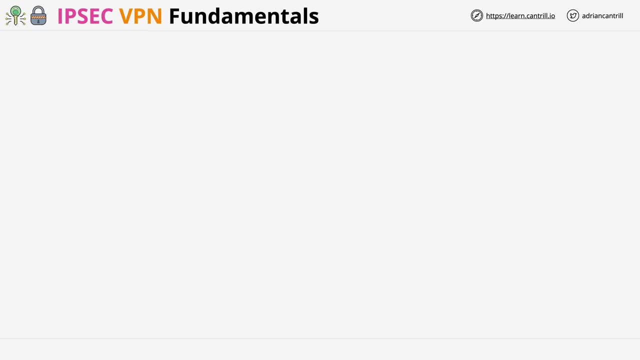 protected. Now, to understand the nuance of what IPsec does, we need to refresh the IPsec. a few key pieces of knowledge. In my fundamental section I talked about the different types of encryption. I mentioned symmetric and asymmetric encryption. Now symmetric encryption is fast. It's. 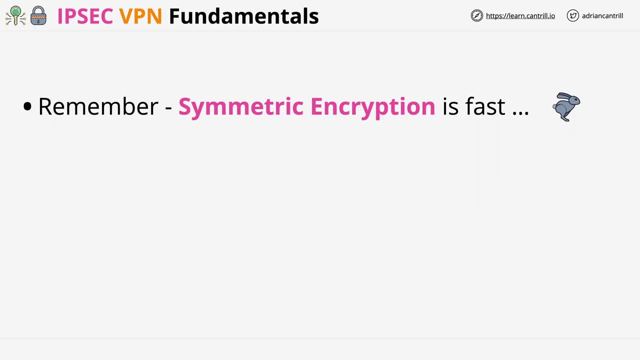 generally really easy to perform on any modern CPU and it has pretty low overhead. But exchanging keys is a challenge. The same keys are used to encrypt and decrypt, So how can you get the key from one entity to another securely? Do you transmit it in advance over a different medium or do you encrypt it? If so, you run. 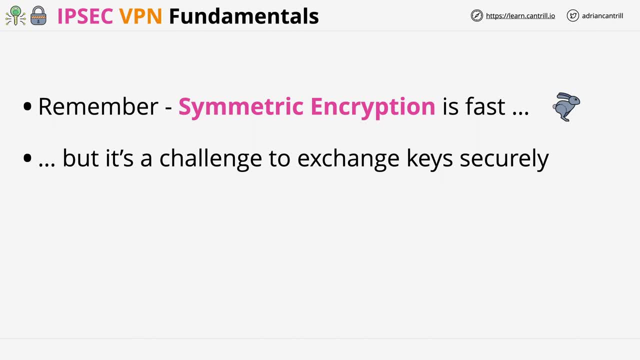 into a catch-22 situation. How do you securely transmit the encrypted key? That's why asymmetric encryption is really valuable. Now. it's slower, so we don't want to be using it all the time, but it makes exchanging keys really simple, because different keys are used for encryption. 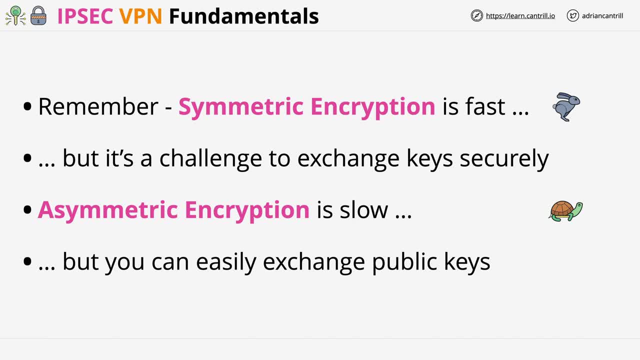 and decryption. Now a public key is used to encrypt data and only the corresponding key is used to encrypt data, and only the corresponding key is used to encrypt data and only the corresponding private key can decrypt that data. And this means that you can safely exchange the public key while keeping the private key private. 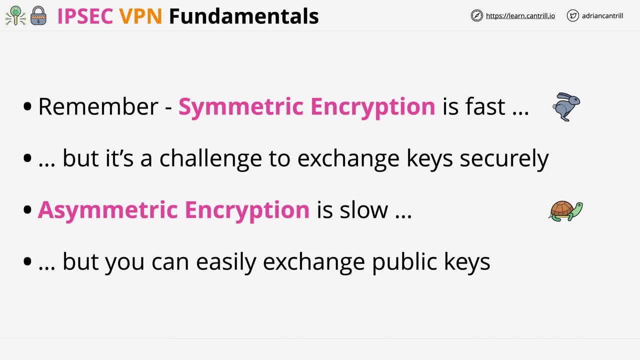 So the aim of most protocols which handle the encryption of data over the internet is to start with asymmetric encryption. use this to securely exchange symmetric keys and then use those for ongoing encryption. Now, I mention that because it will help you understand exactly how IPSec VPN works. 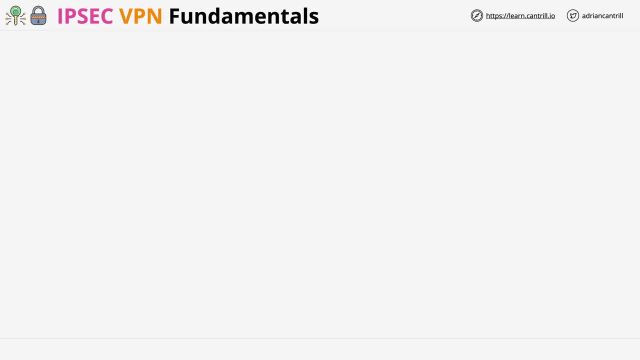 So let's go through it. IPSec has two main phases. If you work with VPNs, you're going to hear a lot of talk about phase 1 or phase 2.. It's going to make sense why these are needed by the end of this lesson. 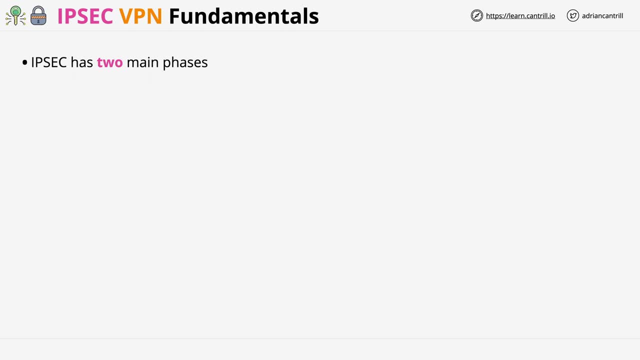 but understand. there are two phases in setting up a given VPN connection. The first is known as Ike phase 1.. Ike, or internet key exchange, as the name suggests, is a protocol for how keys are exchanged In this context within a VPN. There are two versions: Ike version 1 and Ike version 2.. 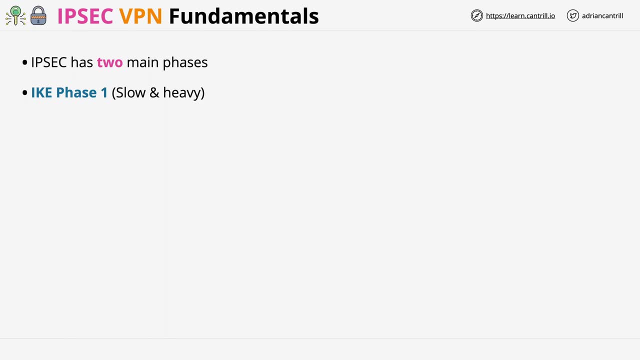 Version 1, logically, is older. version 2 is newer and comes with more features. Now you don't need to know all of the detail right now. just understand that the protocol is about exchanging keys. Ike phase 1 is the slow and heavy part of the process. It's where you initially authenticate. 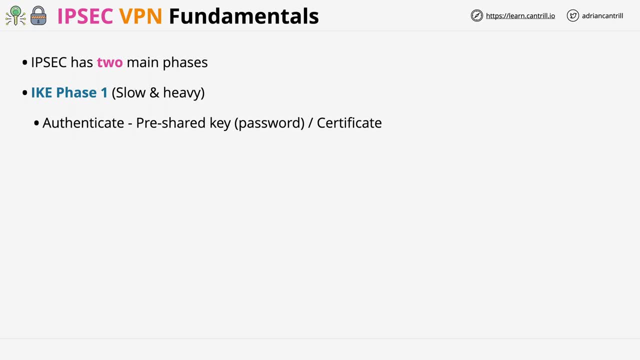 using a pre-shared key, so a password of sorts or a certificate. It's where asymmetric encryption is used to authenticate. It's where you authenticate using a pre-shared key, so a password of sorts or a certificate. It's where asymmetric encryption is used. 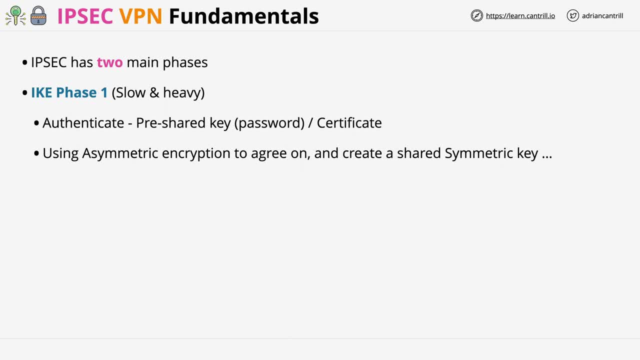 to agree on, create and share symmetric keys which are used in phase 2.. The end of this phase is what's known as an Ike phase 1 tunnel, or a security association known as an SA. There's lots of jargon being thrown around and I'll be showing you how. 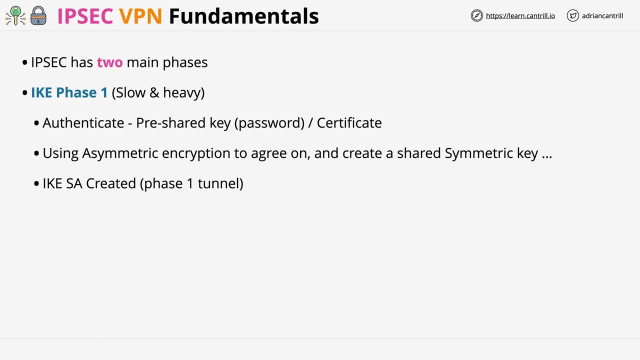 this all works visually in just a moment. but at the end of phase 1 you have a phase 1 tunnel and the heavy work of moving towards symmetric keys which can be used for encryption has been completed. The next step is Ike phase 2, which is faster and much more agile because much of the heavy 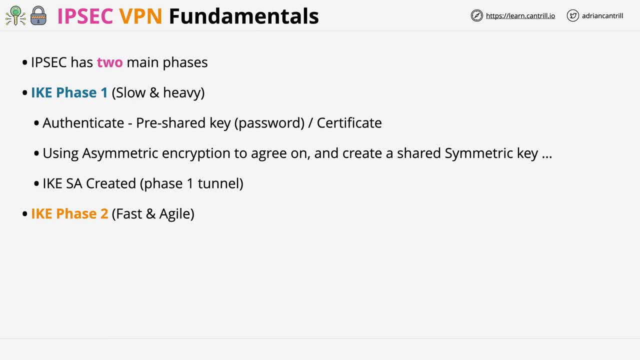 lifting has been done in phase 1.. Technically, the phase 1 keys are used as a starting point for phase 2.. Phase 2 is built on top of phase 1 and is concerned with agreeing encryption methods and the keys used for the bulk transfer of data. 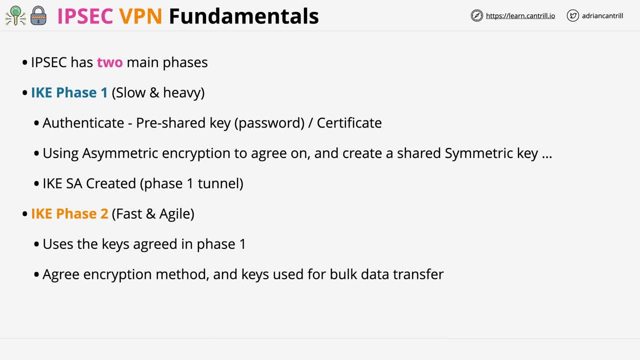 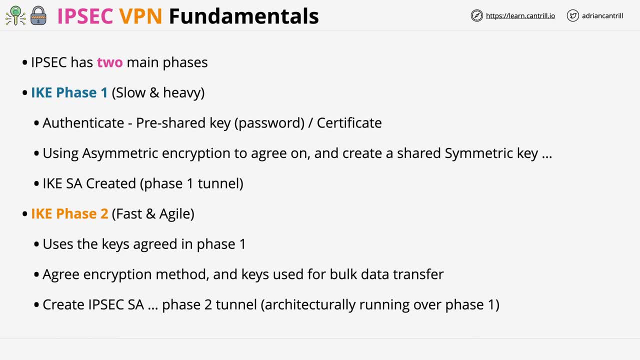 The end result is an IPSec security association, a phase 2 tunnel which runs on a security association. Now, the reason why these different phases are split up is that it's possible for phase 1 to be established, then a phase 2 tunnel created, used and then torn down where no. 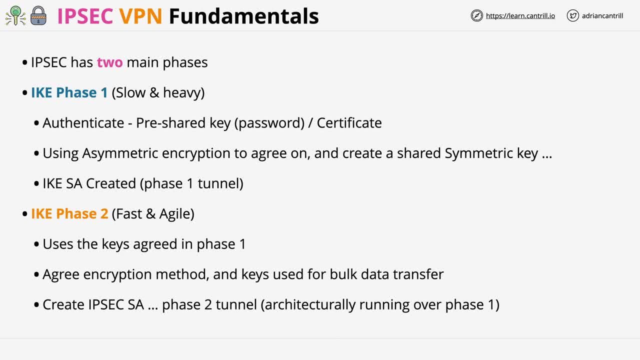 more interesting. traffic occurs, but the phase 1 tunnel stays. It means that establishing a new phase 2 tunnel is much faster and less work. It's an elegant and well designed architecture, So let's look at how this all works together visually. Phase 1 tunnel. 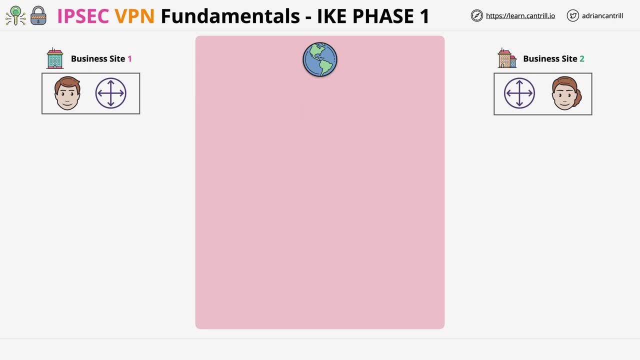 is Ike, phase one. The architecture is a simple one: Two business sites, site one on the left with a user Bob, and site two on the right with a user Julie, and in the middle, the public internet. The very first step of this process is that the routers, the two peers at either side of this. 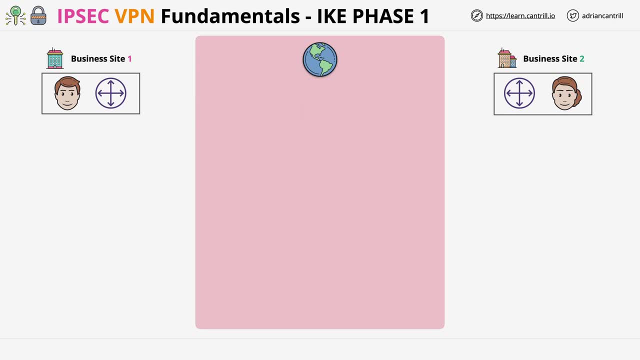 architecture, need to authenticate, Essentially prove, their identity, which is done either using certificates or pre-shared keys. Now it's important to understand that this isn't yet about encryption. It's about proving identity, Proving that both sides agree that the other side should. 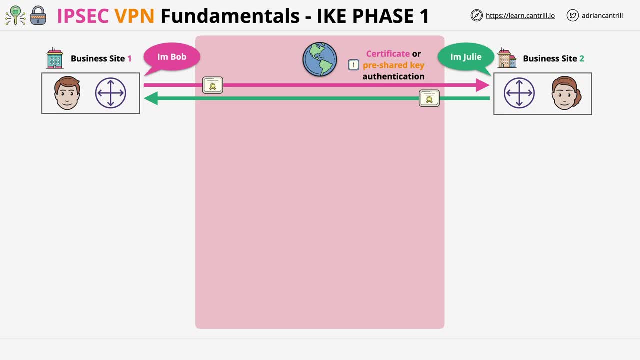 be part of this VPN. No keys are exchanged, It's just about identity. Once the identity has been confirmed, then we move on to the next stage of Ike, phase one. In this stage we use a process called Diffie-Hellman key exchange. Now again, I'm sorry about the jargon, but try your best to. 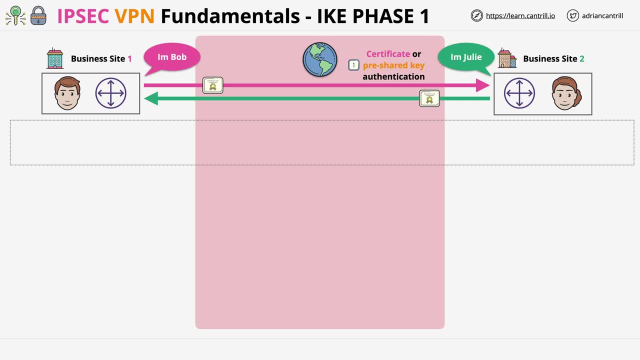 remember Diffie-Hellman, known as DH. What happens is that each side creates a Diffie-Hellman private key. This key is used to decrypt data and to sign things. You should remember this from the encryption fundamentals lesson. In addition, each 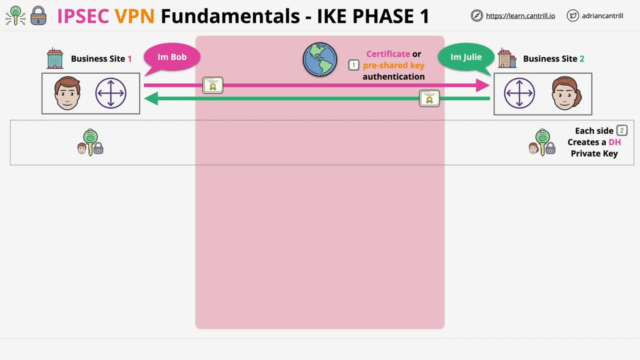 side uses that private key and derives a corresponding public key. Now the public key can be used to encrypt data that only that private key can decrypt. So at this point, each side has a private key as well as a corresponding public key. At this point, these public keys are exchanged. So Bob has 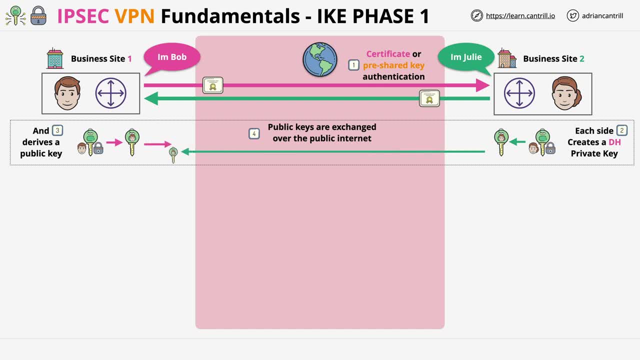 Julie's public key and Julie has Bob's public key. Remember, these public keys are not sensitive and can only be used normally to encrypt data for decryption by the corresponding private key. The next stage of the process is actually really complicated mathematics, but at a fundamental level. 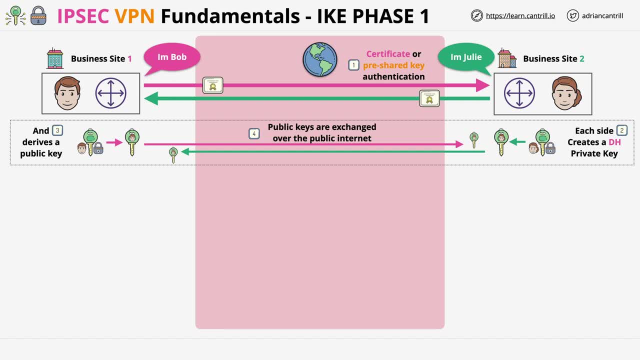 each side takes its own private key and the public key takes its own private key. So Bob takes the public key of the other side and uses this to derive what's known as the Diffie-Hellman key. This key is the same at both sides, but it's been independently generated. Now again the maths. 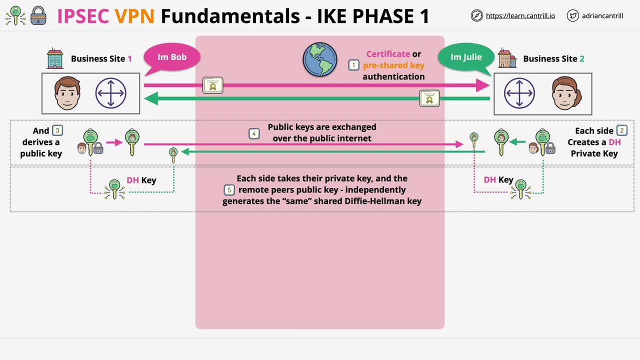 is something that's well beyond this lesson, but it's at the core of how this phase of VPN works And at this point it's used to exchange other key material and agreements. This part you can think of as a negotiation. The result is that each side again is a private key and the public key is the. 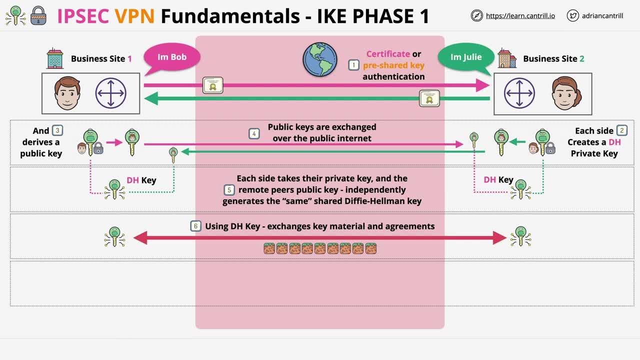 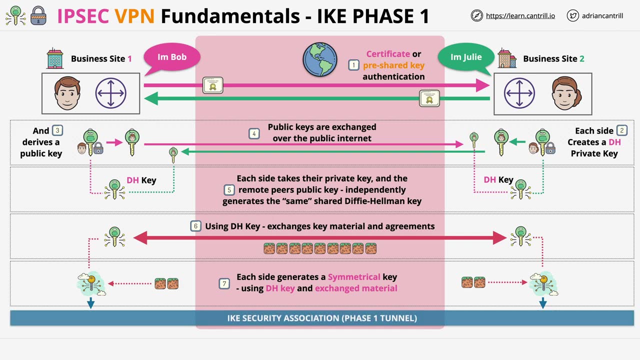 independently uses this DH key plus the exchanged key material to generate a final phase one symmetrical key. This key is what's used to encrypt anything passing through the phase one tunnel known as the Ike Security Association. Now, if that process seems slow and heavy, that's because it is. 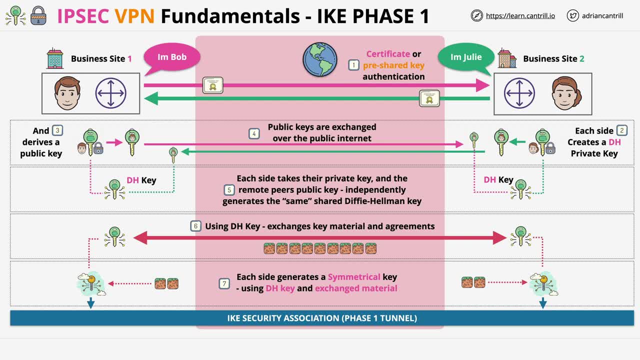 It's both complex and, in some ways, simplistically elegant at the same time, but it means that both sides have the same key. So Bob takes the public key and uses it to derive what's known as the same symmetric key, without that ever having been passed between them, And the phase ends with this. 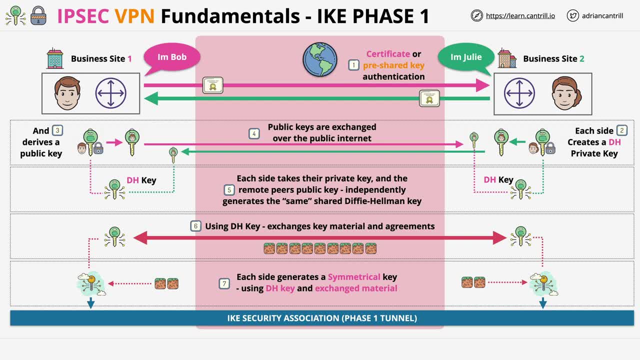 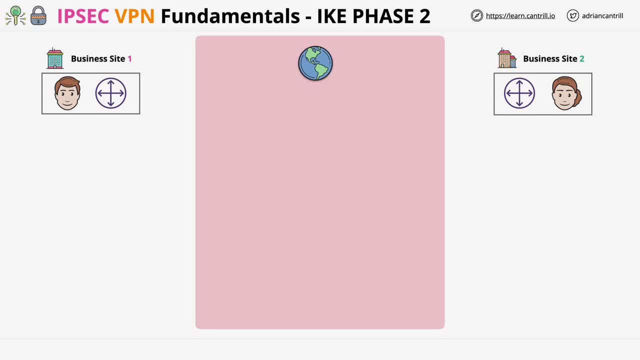 security association in place, and this can be used at phase two. So let's talk about that next. So in phase two we have a few things: First, a DH key on both sides and the same phase one symmetric key, also on both sides, and then finally, the established phase one tunnel During this. 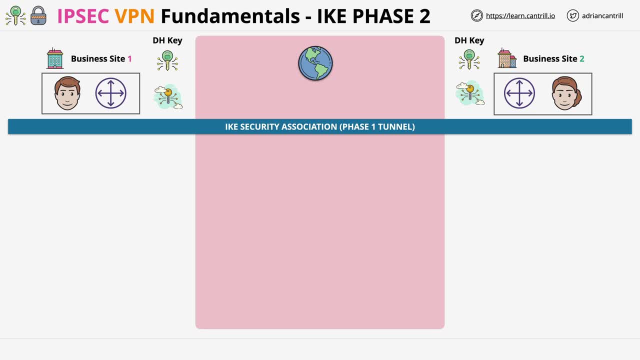 phase. both sides have the same symmetric key and the same phase one tunnel. So in this case, the of the peers are wanting to agree how the VPN itself will be constructed. The previous phase was about allowing this, exchanging keys and allowing the peers to communicate This phase, so Ike phase two. 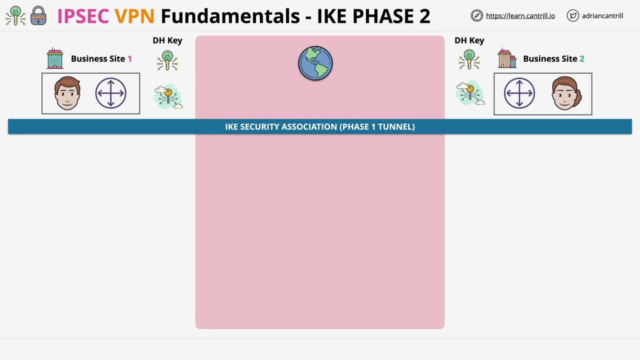 is about getting the VPN up and running, being in a position to encrypt data, So agreeing how, when and what. So the first part of this is that the symmetric key is used to encrypt and decrypt agreements and pass more key material between the peers. So the first part of this is that the 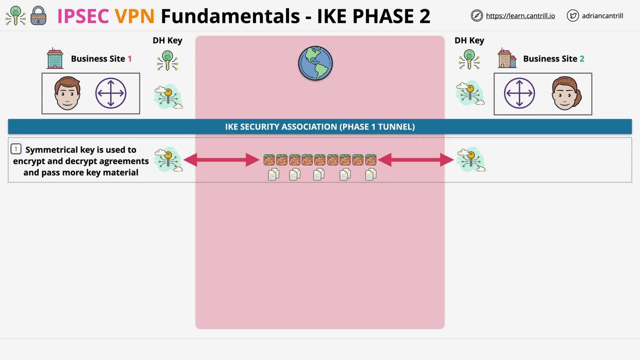 The idea is that one peer is informing the other about the range of cipher suites that it supports- Basically encryption methods- which it can perform. The other peer- in this example the right one- will then pick the best shared one, So the best method which it also supports, and it will let 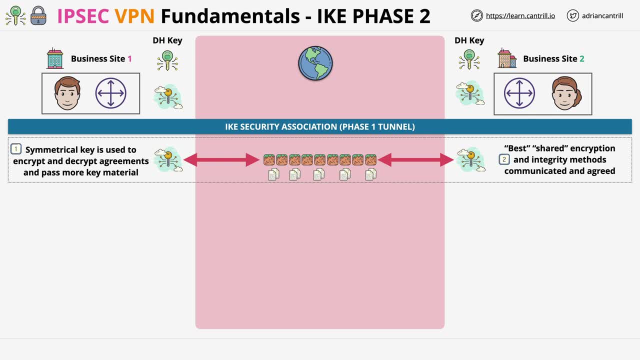 the left peer know, And this becomes the agreed method of communication. Next, the DH key and the key material exchanged above is used to encrypt and decrypt data. So the first part of this is that the key material exchanged above is used to create a new key, A symmetrical IPsec key. This is a key which is 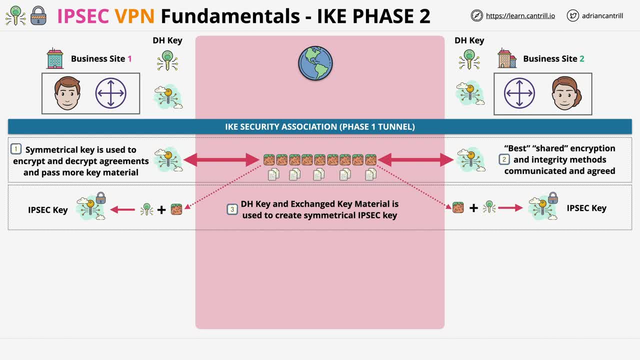 designed for large scale data transfer. It's an efficient and secure algorithm, And the specific one is based on the negotiation which happened above in steps one and two of this phase. So it's this key which is used for the encryption and decryption of interesting traffic across the VPN tunnel. 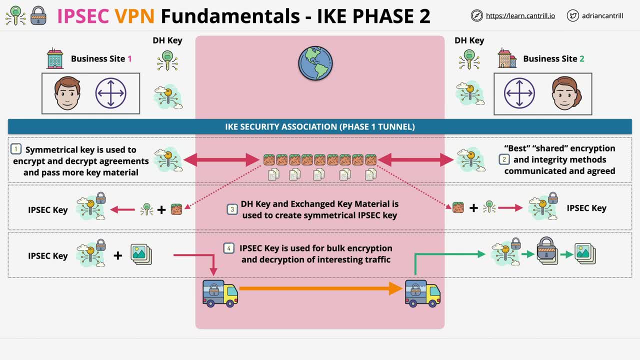 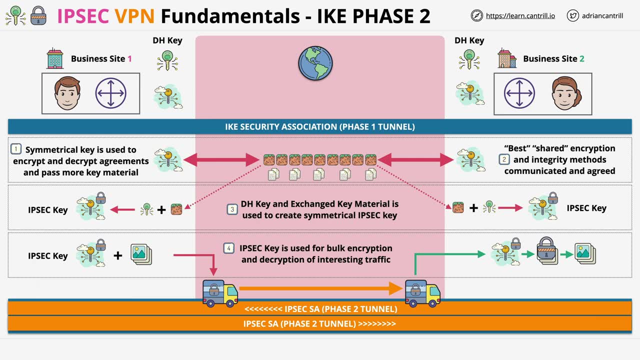 Across each phase one tunnel. you actually have a pair Of security associations, One from right to left and one from left to right, And these are the security associations which are used to transfer the data between networks at either side of a VPN. Now, there are actually two different types of VPN which you need to understand: Policy based VPNs. 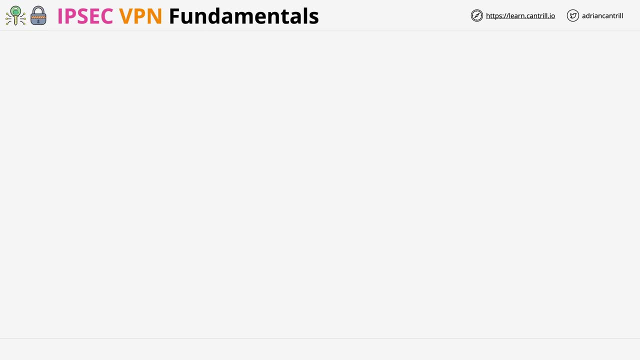 and route based VPNs. The difference is how they match interesting traffic. Remember, this is the traffic which gets sent over a VPN. So with policy based VPNs, there are rules created which match traffic And, based on this rule, traffic is sent over a pair of security associations, One which is used for each direction of traffic. It means that you 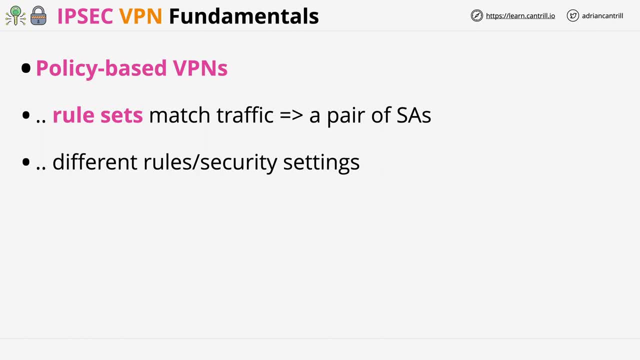 can have different rules for different types of traffic, Something which is great for more rigorous security environments. Now the other type of VPN are route based VPNs, And these do target matching based on prefix. For example, send traffic for 192.168.0.0, slash 24 over this VPN With this type. 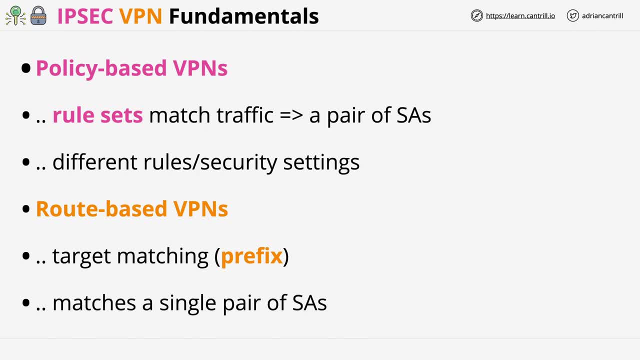 of VPN, you have a single pair of security associations for each network prefix. This means all traffic types between those networks use the same pair of security associations. Now, this provides less functionality, but it is much simpler to set up. To illustrate the differences: 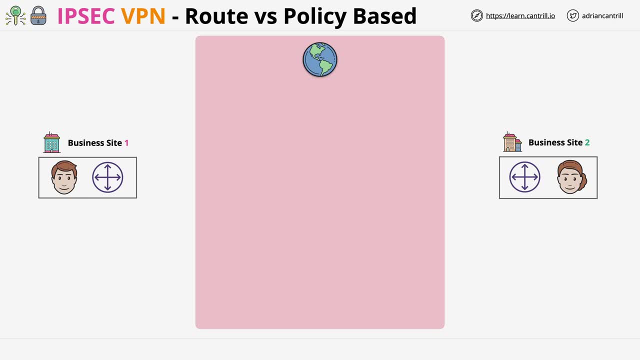 between route-based and policy-based VPNs. it's probably worth looking visually at the phase 1 and phase 2 architectures. Let's start with a simple route-based VPN. The phase 1 tunnel is established using a phase 1 tunnel key. Now, assuming that we're using a route-based VPN, 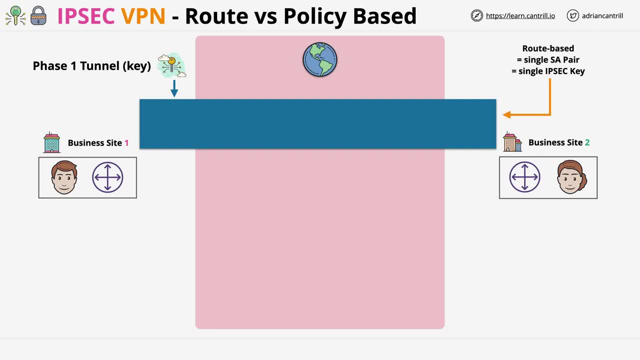 then a single pair of security associations is created, one in each direction using a single IPsec key. So this means that we have a pair of security associations, essentially a single phase 2 tunnel running over the phase 1 tunnel, That phase 2, or IPsec tunnel, which is how we talk.